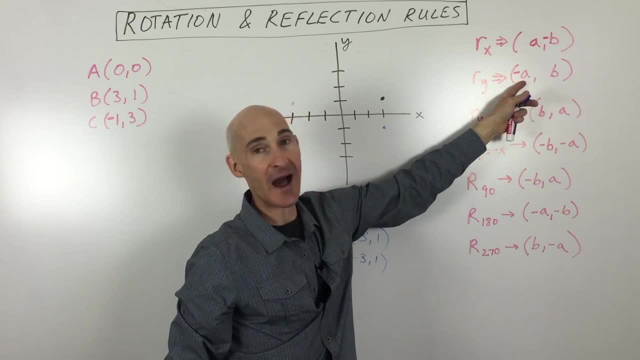 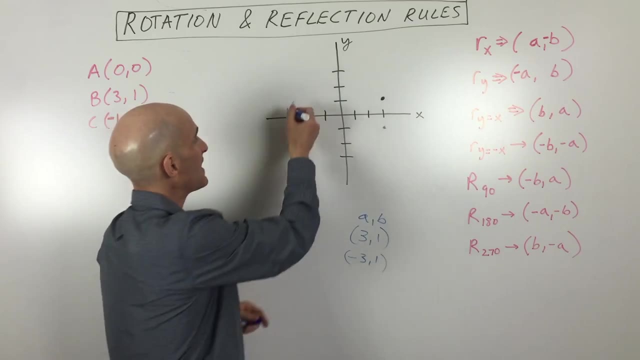 reflect over the y-axis, it's the x-coordinate that's going to be the opposite sign. So if it's positive, it'll become negative, If it's negative it'll become positive, But the y-coordinate will stay the same. You can see this is at the same height. Okay, it's at the same y-value Now. 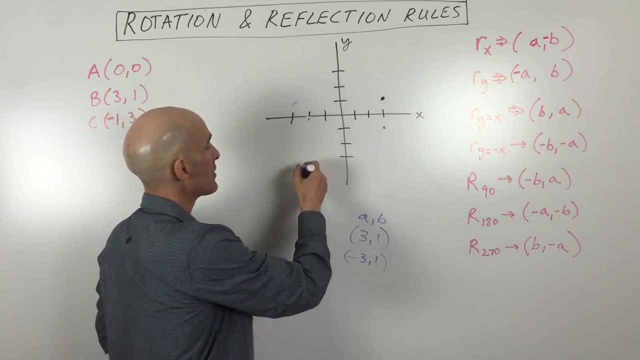 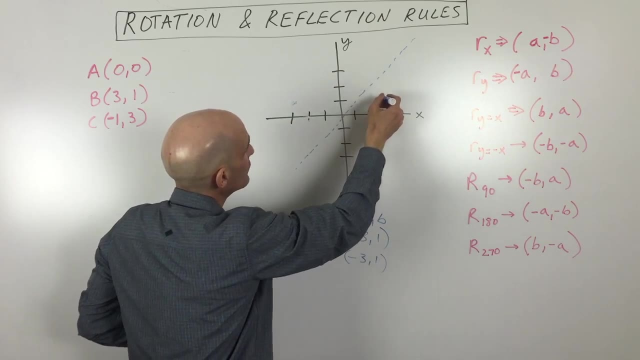 if you reflect over the line y equals x, y equals x. is this line here on a 45-degree angle? It has a slope of 1, like that, If you take this point and you fold it over this line. okay, you want to? 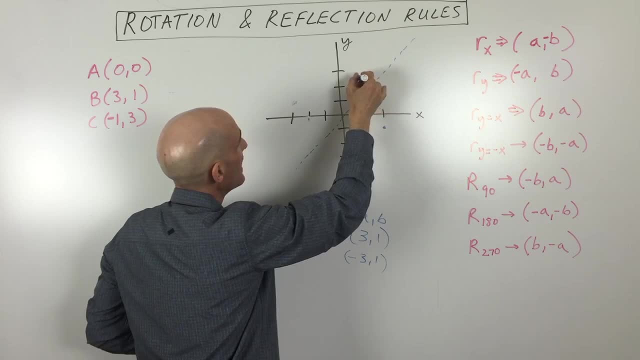 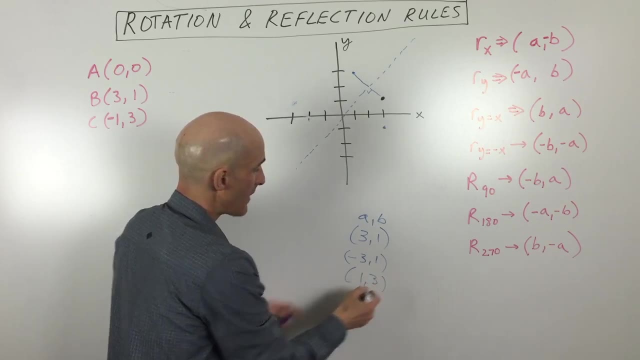 measure the perpendicular distance to that line If you go the same distance on the other side. okay, right there you can see you're going to be at 1, 3 now. Okay, so what happened to go from 3,? 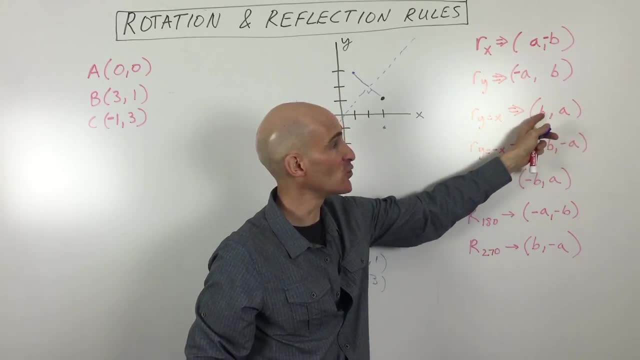 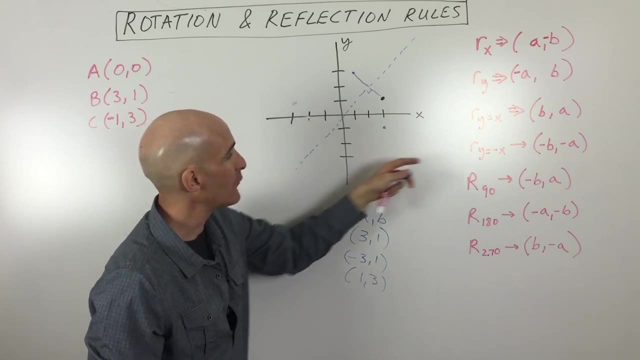 1 to 1, 3?. Well, you can see what we did is we actually switched the x and the y coordinates. It reflects it over. this line y equals x. Now, if we look at the line y, equals negative x, that's. 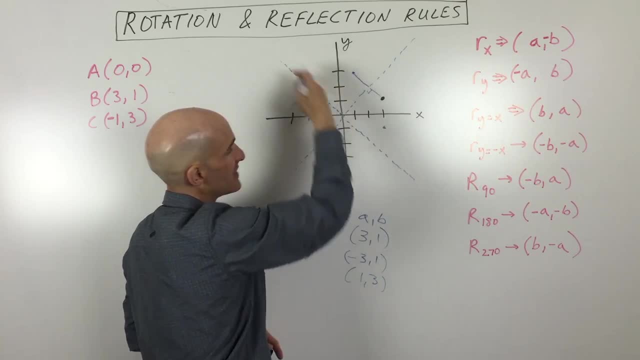 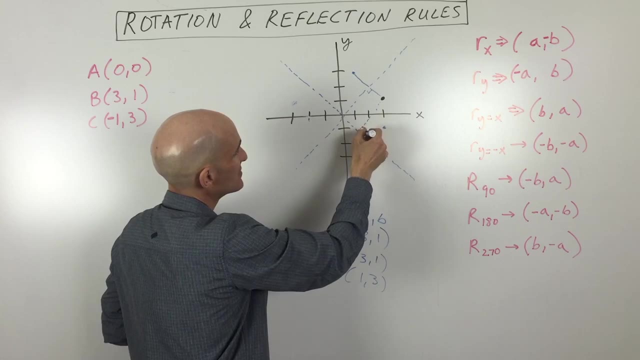 a line with a negative 1 slope. Okay, it's going down at this angle on a 45-degree. Okay, and you can see here, when you reflect over this line again, you want to measure that perpendicular distance to the line. You want to go the same distance on the other side, okay, of that line. 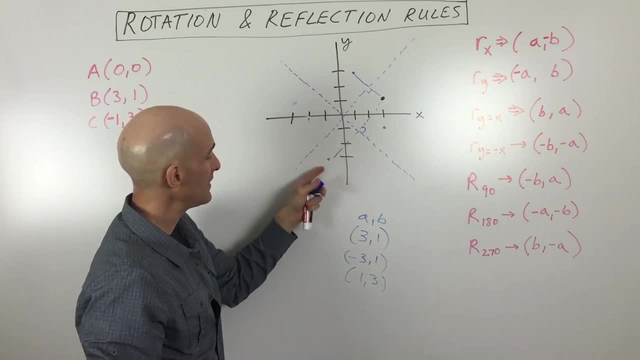 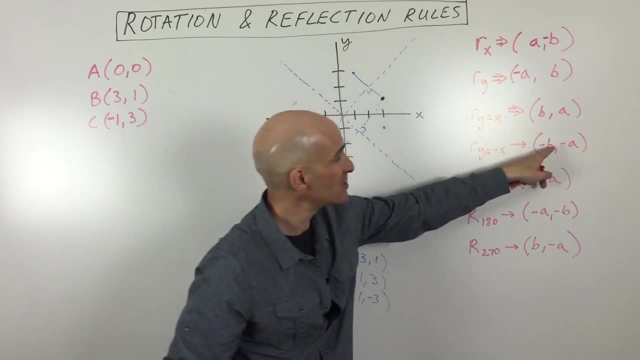 Okay, and you can see the new coordinates are going to be negative 1, negative, 3, negative 1, negative 3.. So what happened there? We went from 3, 1 to negative 1, negative 3.. We switched the x and the y coordinates. okay. 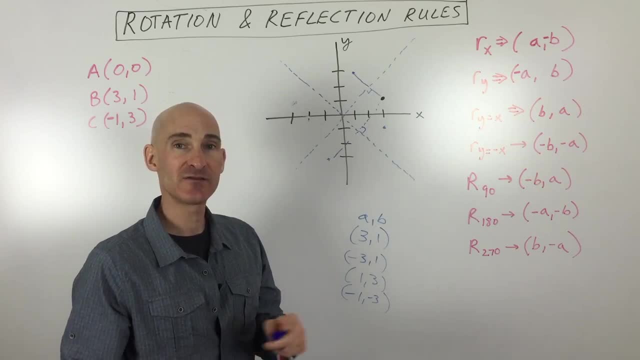 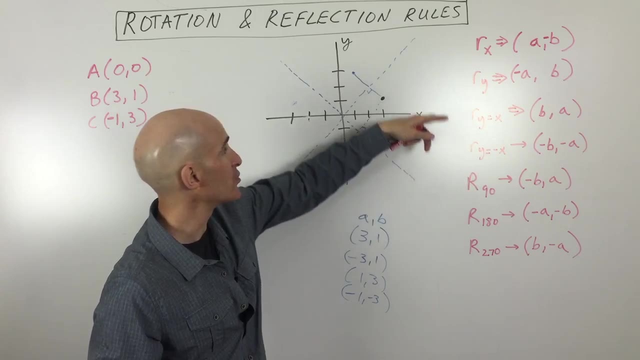 And we made them the opposite signs. So if they were positive, we make them negative, If they were negative, we make them positive. okay, Now, the capital Rs here, you can see, are for rotations, So that's for when you're turning. Now, imagine if you pick this up and you rotate. 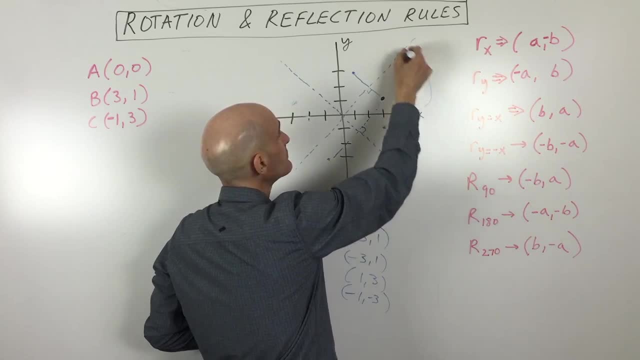 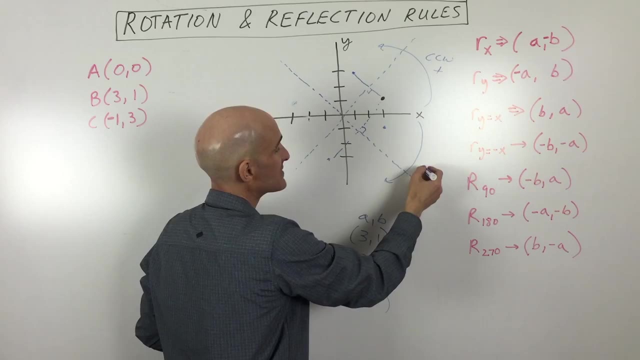 it and you turn it, And the important thing to remember is that when you're turning it counterclockwise, that's actually the positive direction. When you turn it clockwise, that's actually the negative direction. Okay, so we're going to be going counterclockwise. 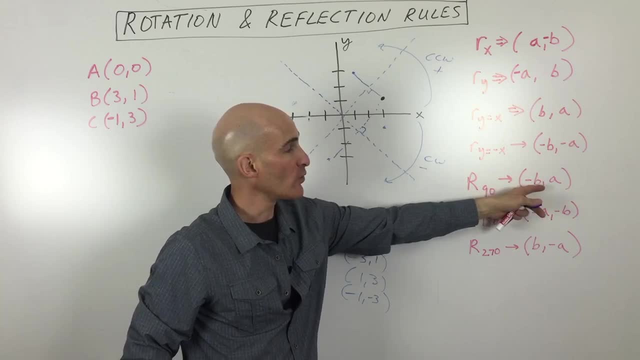 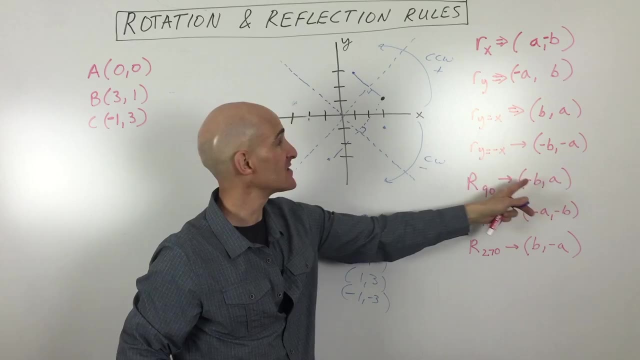 Okay, and so if we want to rotate 90 degrees, what we do is we take the x and the y coordinates, we switch them and we make the new x coordinate the opposite sign. So for 3,, 1, what we're going? 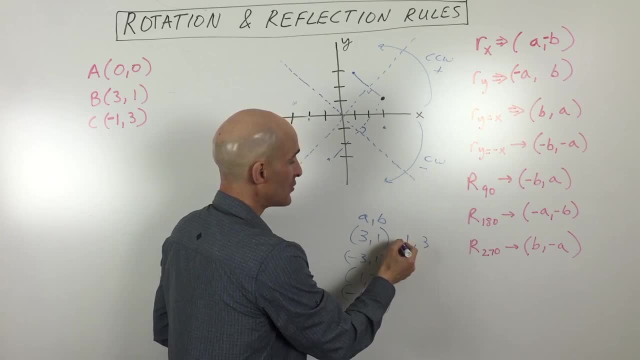 to do is we're going to switch them, So it's going to be 1, 3, but now we're going to make the new x coordinate the opposite, So this point here should be at negative 1, 3.. Now I was telling. 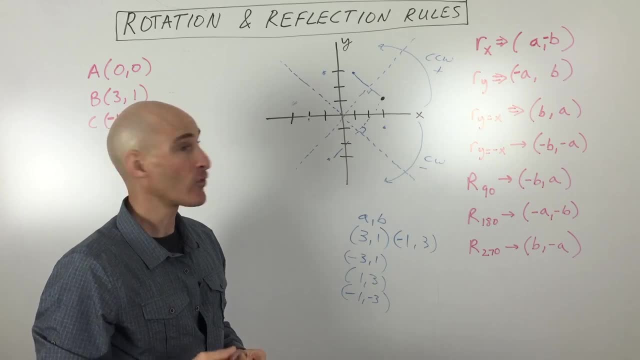 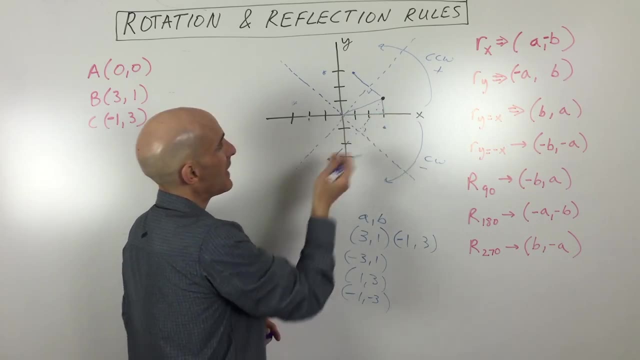 you at the beginning of the video. I wanted to show you some ways to remember these formulas in case you forget, and what I usually do is I draw a triangle. I make a triangle like this, okay, and I think about pivoting at the origin. So I'm rotating this triangle Now look what happens now. 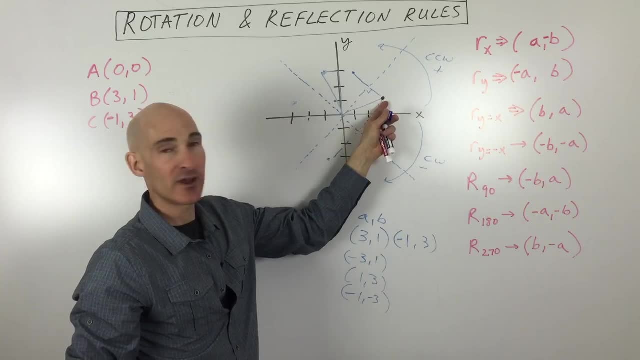 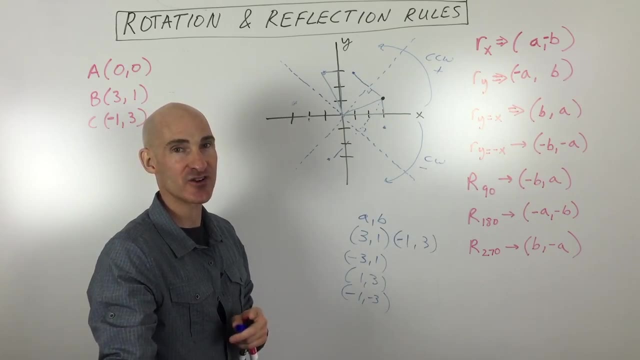 Okay, can you see the new triangle? So if you take a simple example like 3, 1, like that, don't pick the numbers, so they're exactly the same, the coordinates, so they're exactly the same. Pick one so that you know it's larger. 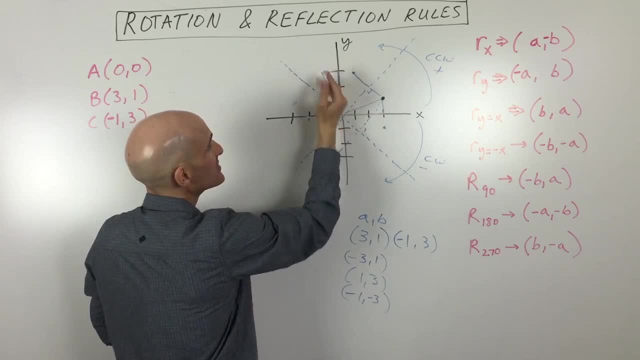 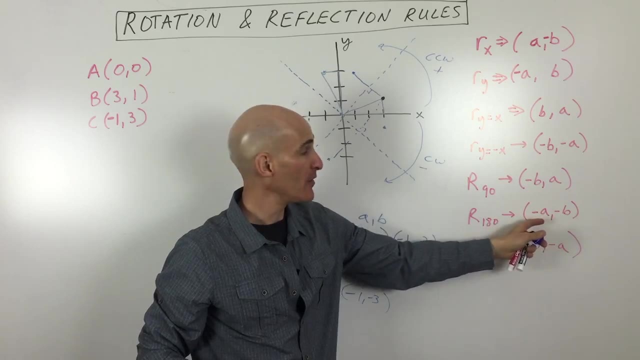 Then the other one, and you'll be able to see this illustration a little bit better. You can see what's happening Now. if we rotate 180 degrees, the x and the y coordinate are going to stay in the same spot, right, but they're both going to be the opposite sign. So for 3,, 1,, that's going to. 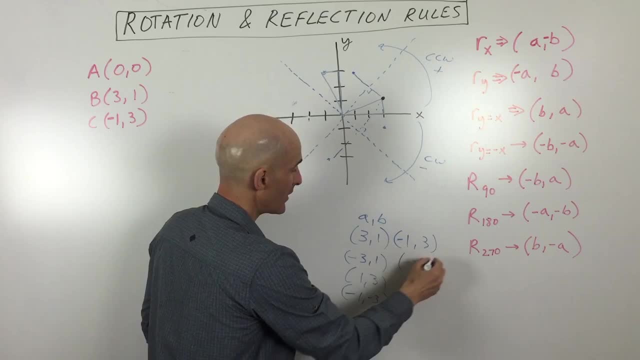 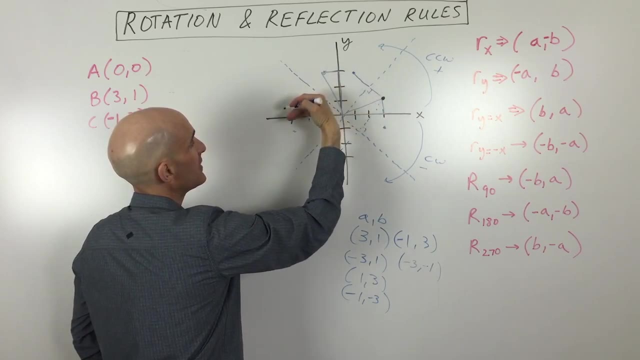 become negative 3,, negative 1, and let's see if that makes sense- Left 3,, down 1.. Again, if we're using our triangle illustration, if we rotate this 180 degrees, which is a half turn, there you go. 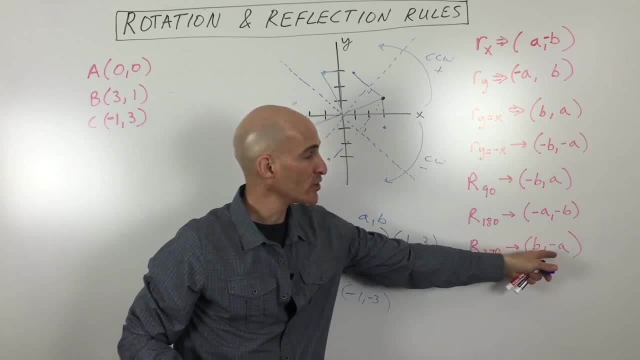 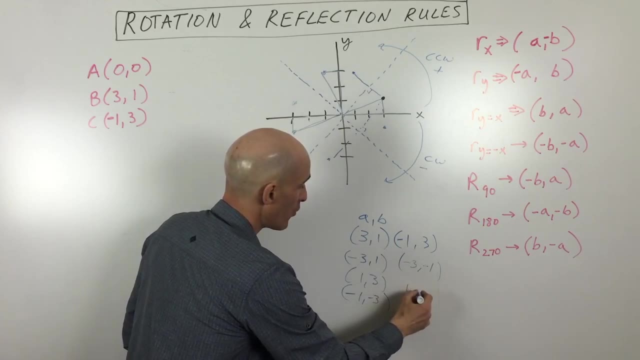 So you're right there: 270 degrees. what you do is you switch the x and y coordinates again, but now you're making the y coordinate the opposite sign. So if we switch these 1 and 3, we're making the. 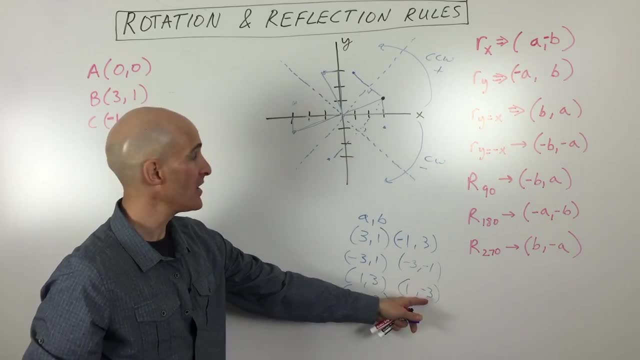 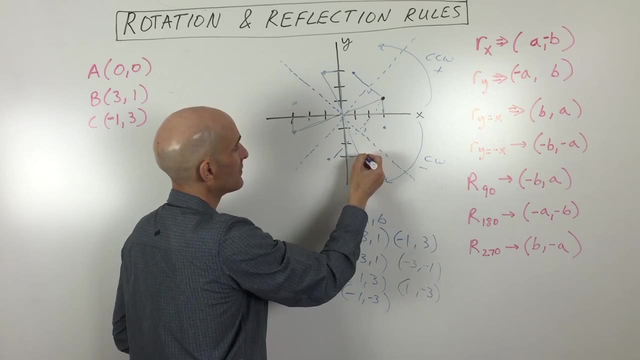 new y, coordinate the opposite, sign the new one. okay, So this is going to be at 1, negative 3, right here and again. if you look at that triangle you can see right there. So it's just like rotating 90,, 180,, 270,. there's the location of your new point, right there.